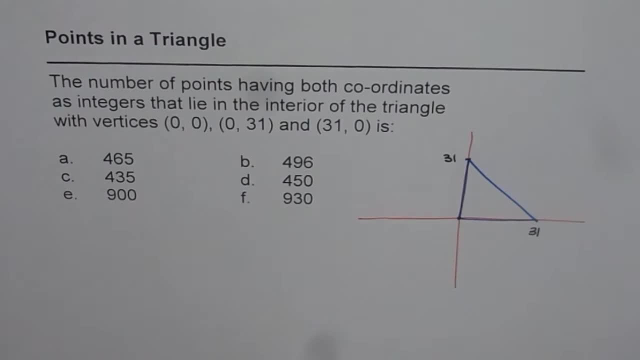 Like 0, 0, 0,, 31,, 31, 0 are integers, right, So we need these kinds of integers. How many of them are within the boundary of this triangle? So we have to exclude the points which are on them. Do you understand When we say inside? 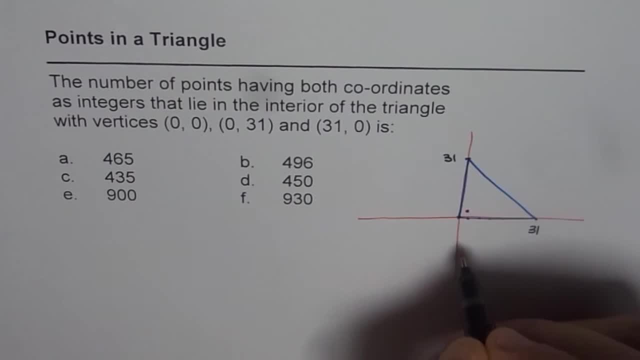 then the very first point will be, which is inside the triangle. So let's understand that right Inside means we are excluding the points which are on the boundary right. So, and then the next will be right. Then we'll have, likewise, The last point. 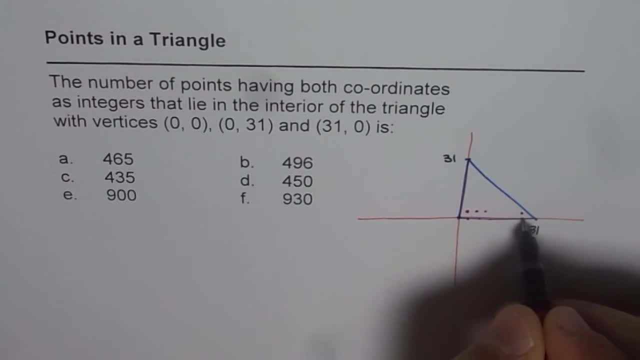 inside will be what? If I move one step then on this it should be 31.. And 30 and 1 will be on the hypotenuse of this triangle. Let's to be very clear. let's find the equation of this hypotenuse. What is the equation of? 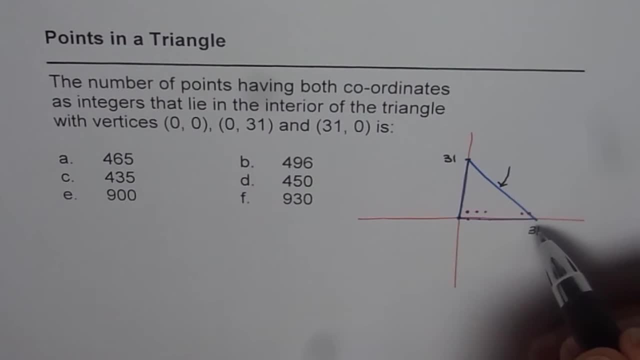 this line? Well, this line has a slope of negative 1, right y is minus 31 and x is 30. So slope is negative 1. And the y-intercept for this line is 31.. Therefore we can write. 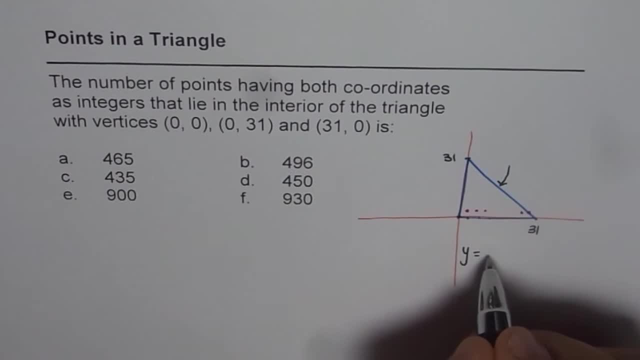 down the equation of this line as y equals to minus x plus 31,. right, So that becomes the equation of this line. So basically, the sum of x and y points, which is x plus y, is basically 31,, right? If my coordinate point is 30 for x, then 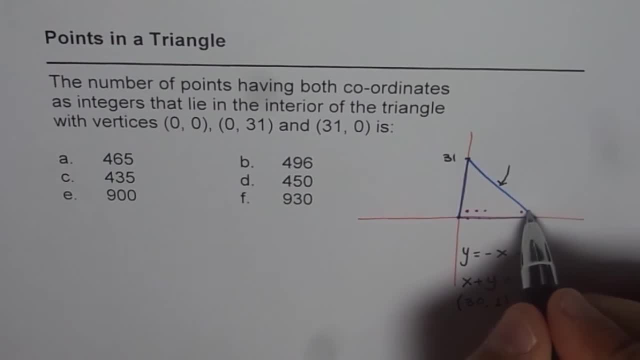 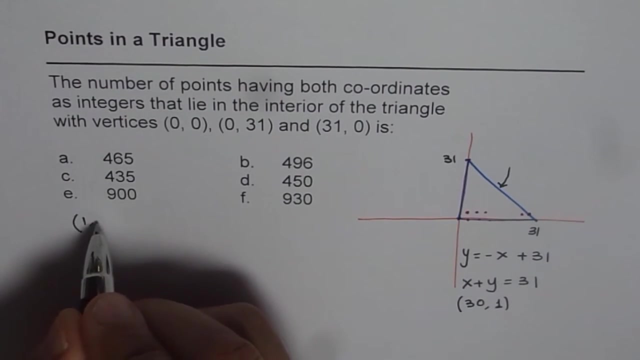 y will be 31.. And this point will lie on the hypotenuse right. So how many points do I have inside? In the very first row, I have 29 points right, Starting from 1, 1, 2, 1, 2, 2,. sorry, 2, 1, I should have written, Well, 1,. let me say now vertical points, since 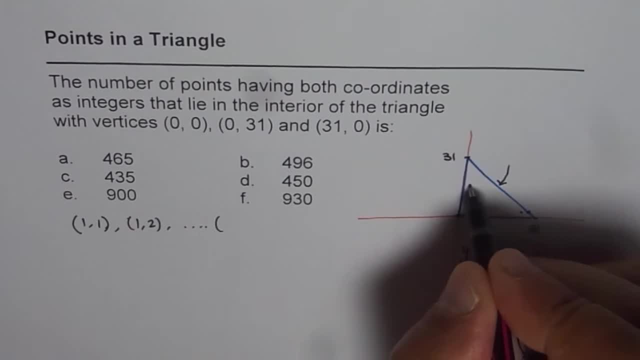 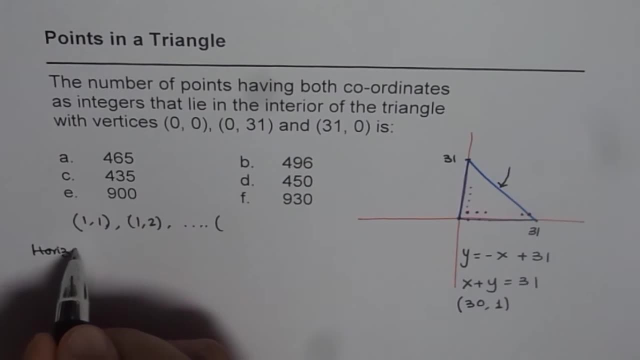 I wrote 1.. If you go up like this, In that case those are the points, But let us see horizontal points first. So horizontal points will be 1, 1. And then we will be having 2, 1.. Likewise. 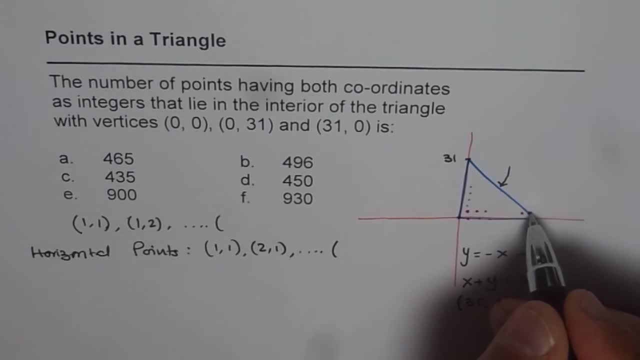 still 30 and 1 will be on the triangles. We'll consider 29,- 1, right, So that means we have 29 points In the first row or the bottom row of this triangle. right, So we have 29 points As. 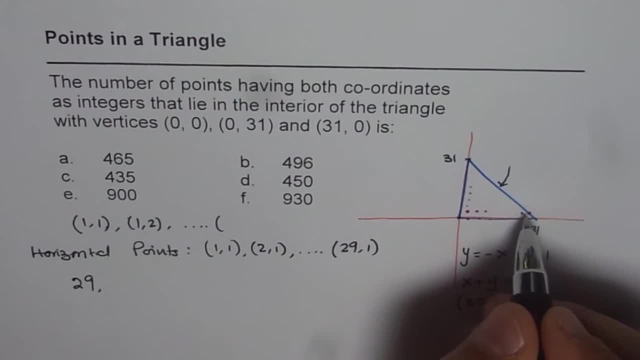 we move up, these number of points are going to reduce. Do you see that? So this point here will be 1,, 2, right, Then it will be 2, 2.. Do you see that? So the y points will. 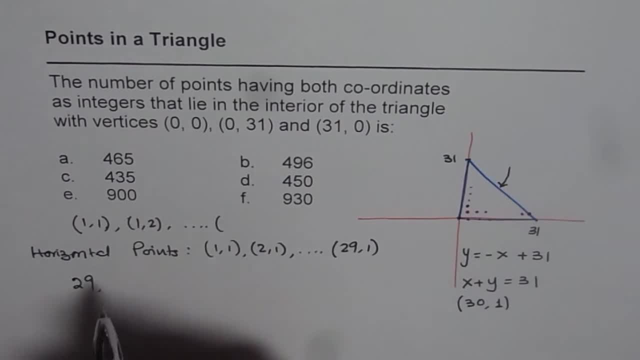 be decreasing, correct, And so we'll have 28 points. So we have 29 points, So the y points will be decreasing, correct, And so we'll have 28 points. 28 points in the next row, And similarly, as we move up, these number of points will. 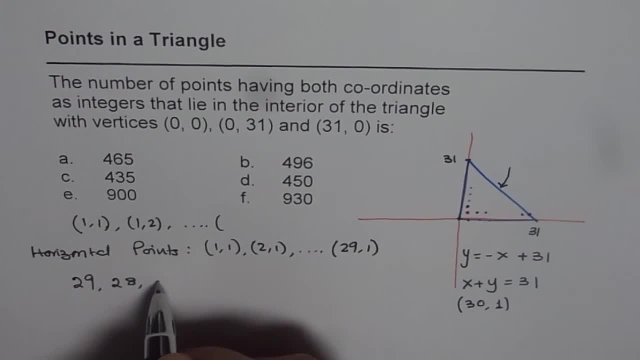 be reducing by 1 each time, So we'll have 28,, 27.. Likewise 3,, 2, and 1.. So these are the number of points within the triangle whose coordinates will be integer values right. Well, as far as the points are concerned, they're infinite number of points, But the 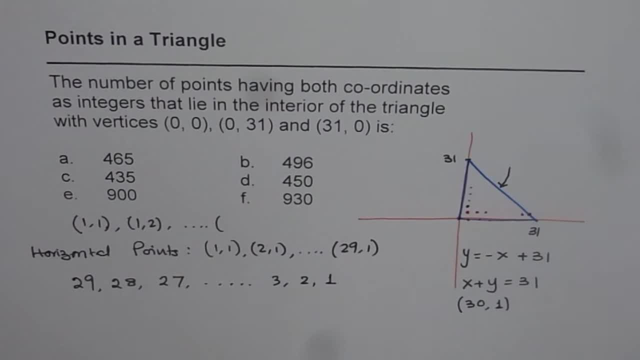 points with integer values, as both x and y coordinates will be these many Sum of these right? So we're trying to find sum of these, So we have to add these numbers up to get our answer right. So that is the whole idea. So sum of first 29 numbers is: 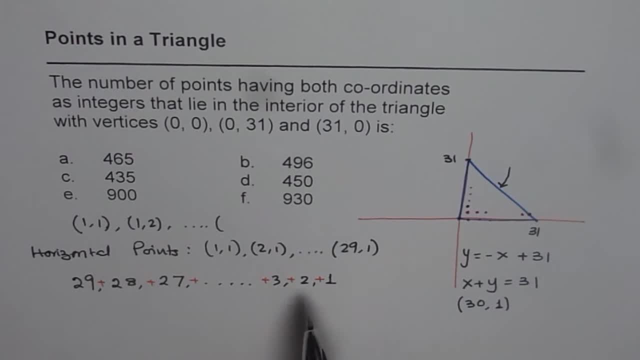 close to our answer, right. So what is the sum of first 29 numbers? One way is use the formula, which is 8.. 8 times n plus 1 divided by 2, right Sum of numbers. That formula can be utilized. 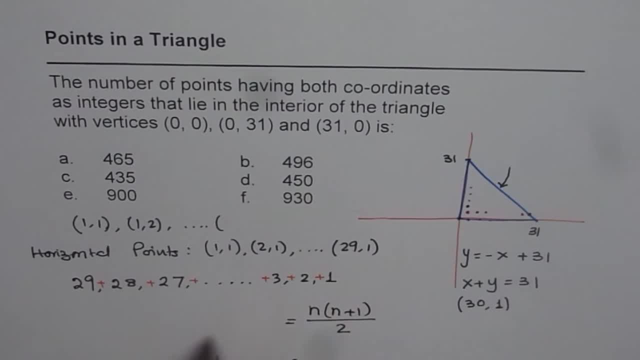 n for us is 29,, right? So we do get 29 times 30 divided by 2 as our answer, right? We could also derive this result. Derive how: If I add 29 and 1, what do I get? I get 30. Do. 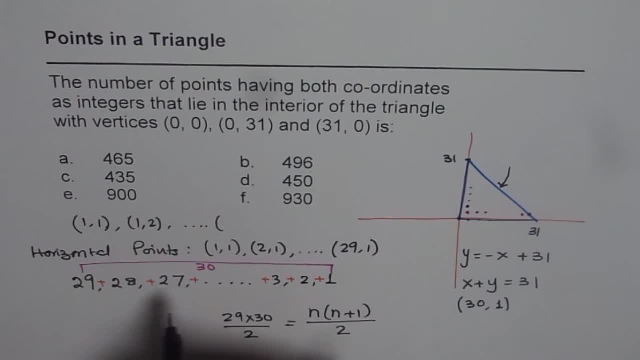 I get 30. if I add 28 and 2, I will again get 30. if I add 27 and 3, I'll get 30 right. so how many of these 30s am I going to get right? 15 of them, half the combinations. do you see that? so there'll be. 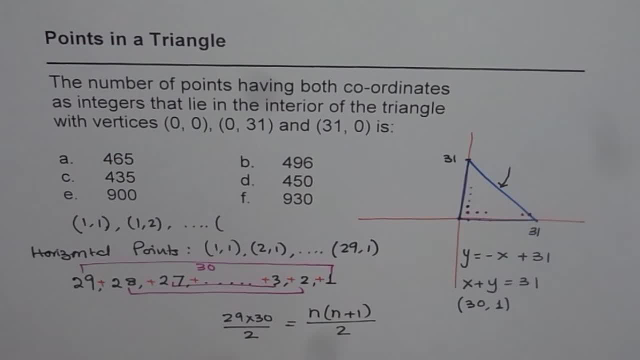 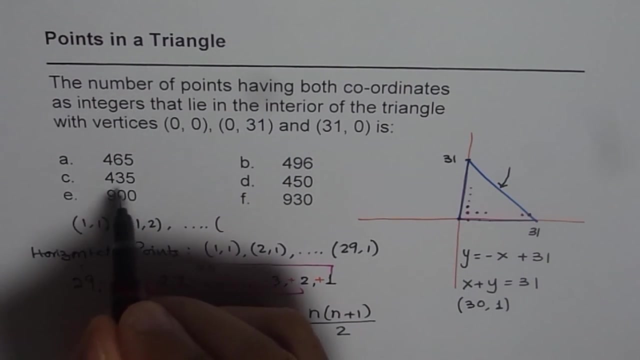 50 combinations of this. so basically, it is going to be as equals to 29 times 15, right? so 29 times 15 is the total number of points which will be inside this triangle, having both x and y coordinates as integer values, right? which is, if you calculate, 435. 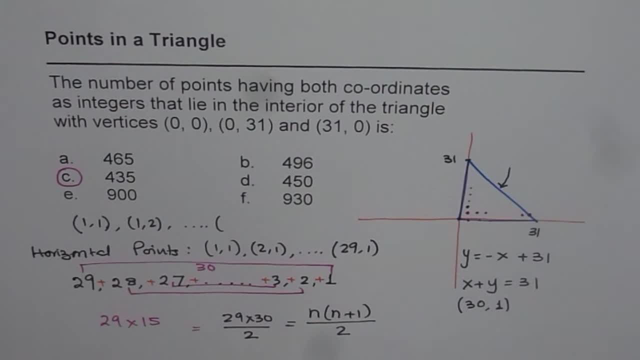 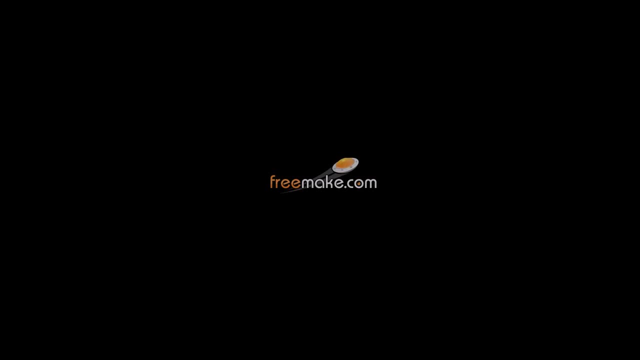 so so that is the answer for this particular question and that is how we derive at it. I hope that makes sense. thank you and all the best you. 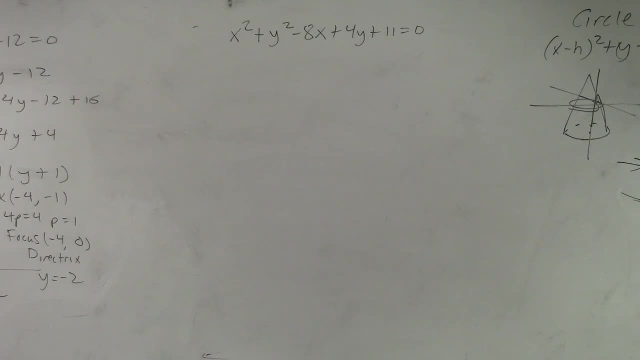 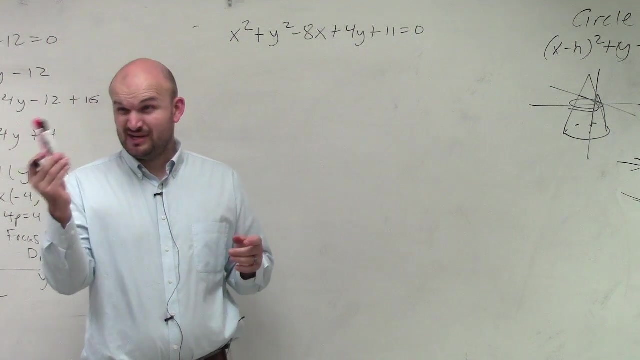 I know we're kind of a little bit time crunched, but I want to huh Yeah. So I'll try to go through as quickly as possible. but I am going to do something that's going to be color coding on this, which will be very, very helpful for those of you that like color coding. And since it is, 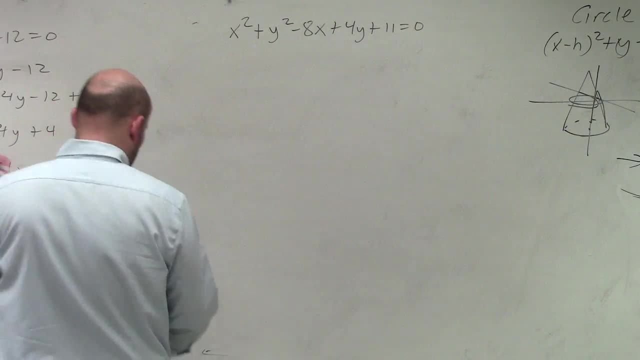 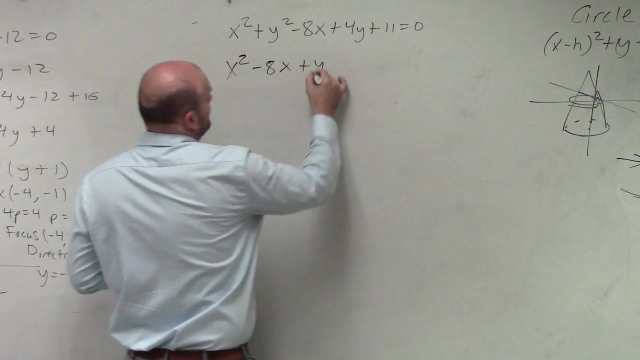 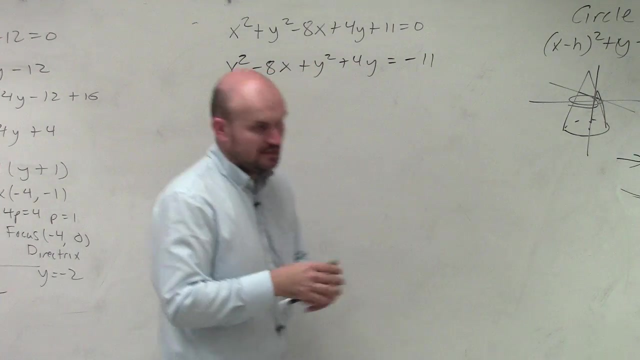 May I'll do Christmas colors, because that makes me think of the wintertime, even though Florida wintertime is not really winter, But anyways. so first thing you guys want to do is group- Let's group- your variables, and everybody see what I did. Okay, Now we need to complete the 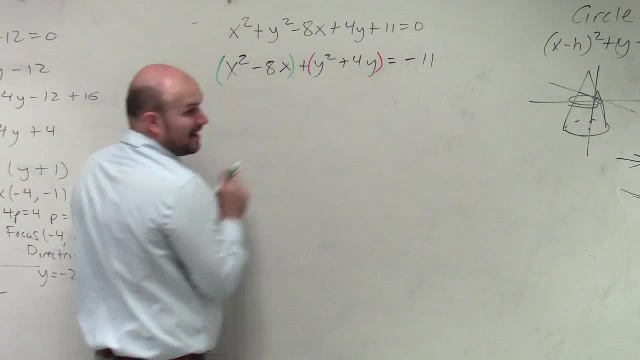 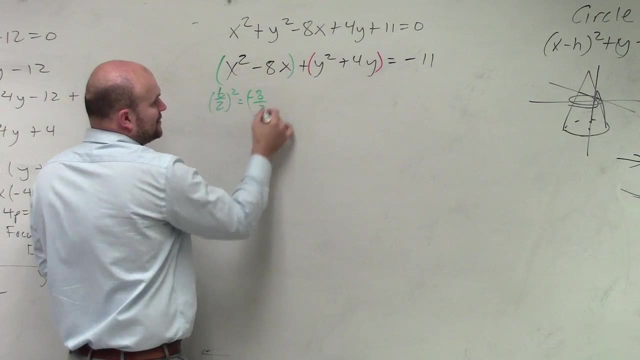 square for the Xs and we need to complete the square for the Ys. So in both of these cases I need to take B divided by two and square it. So in this one it's negative. eight divided by two squared Negative. eight divided by two is negative four Negative four squared is 16..